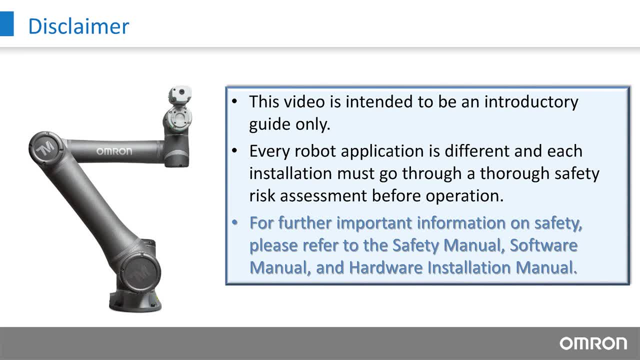 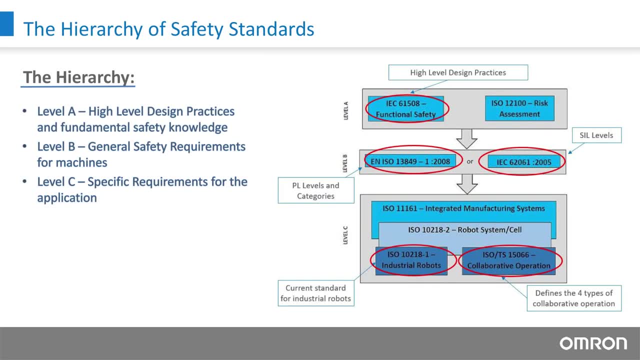 please refer to the Safety Manual, Software Manual and Hardware Installation Manual, Safety Standards and Safety Functions. Here is a slide that shows the hierarchy of the introductions and safety functions. standards that are relevant to the safety of collaborative robot operation. The OMRON TM robots comply with the combined scope of ISO 10218-1 and ISO TS-15066 for human. 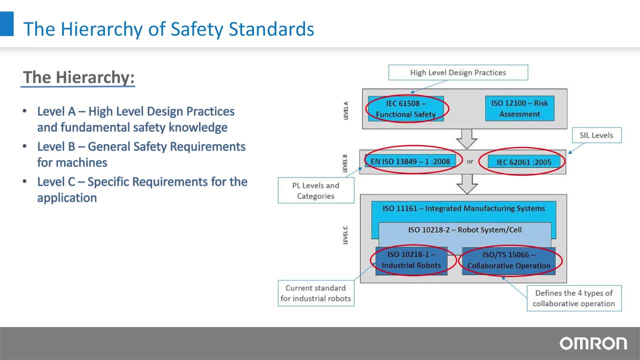 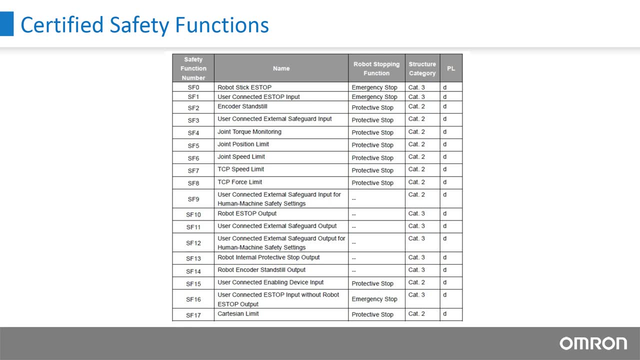 robot co-operational safety, allowing the robot to be programmed with both speed and force limits. Currently, OMRON has 17 certified safety functions that were all certified to be compliant with ISO 13-1.. ISO 13-849-1 defines how a safety-related control system must be designed to achieve. 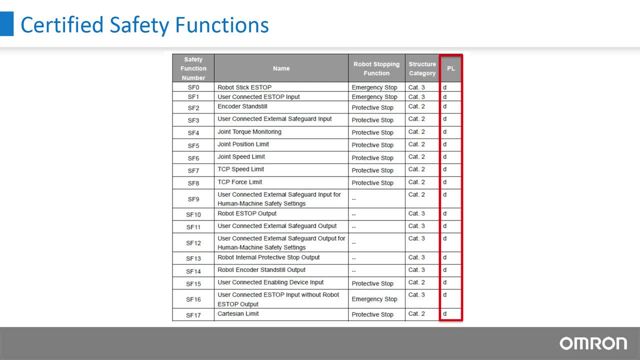 a specific performance level, and performance level D is the second highest reliability classification, meaning that the safety function is reliable. Force and speed monitoring are the defining capabilities of collaborative robots. The safety functions of the OMRON TM robots, including power limit and force limit, are always active and compliant with ISO 13-849-1.. 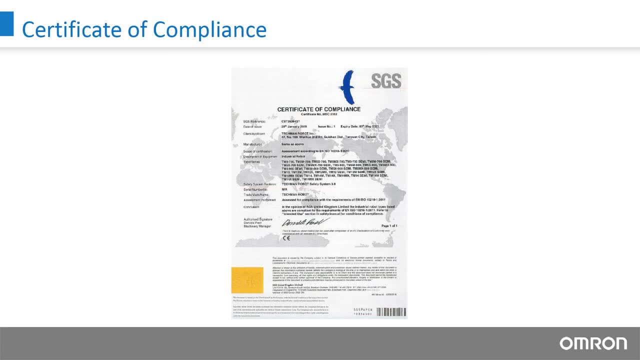 All compliance with safety standards were tested and certified by SGS, an organization based in Switzerland that provides inspection, verification, testing and certification services. The certificates of compliance from SGS can be found in our Safety Manual. Emergency Stop and Protective Stop. Emergency Stop and Protective Stop. 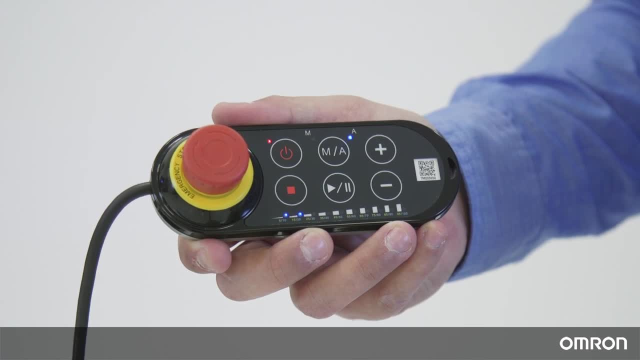 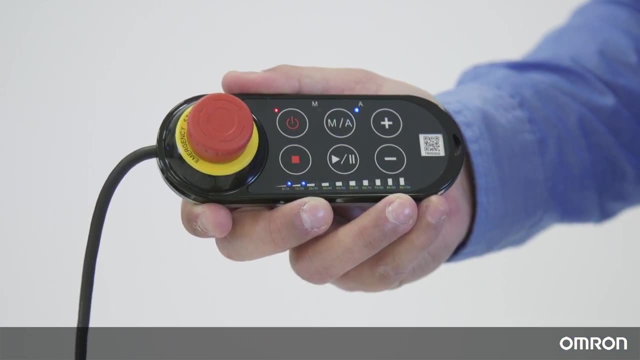 Emergency Stop and Protective Stop. There are two types of safety stops: the Emergency Stop or E-Stop, and the Protective Stop. E-Stop is initiated when a person hits the E-Stop button on the robot stick. When E-Stop is initiated, the robot will make a safe stop and then the power will be removed. 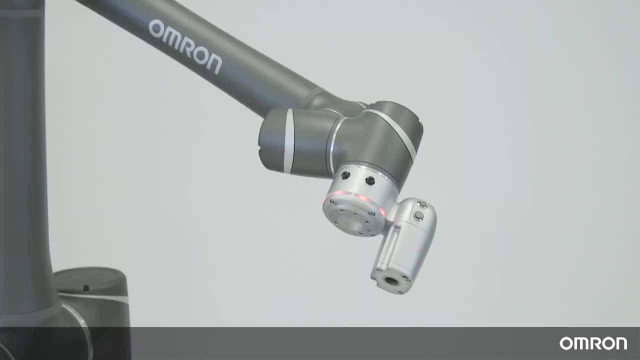 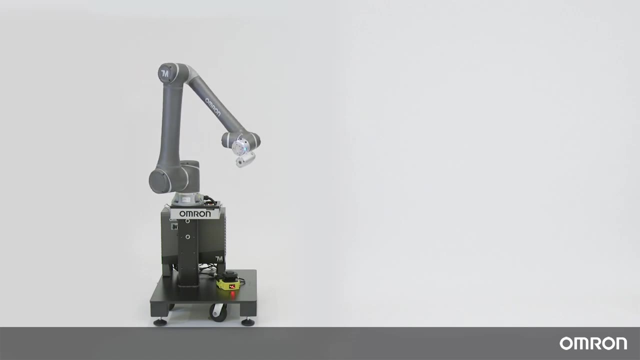 You will have to recover the robot from E-Stop before it can go back to operation. Meanwhile, a Protective Stop is a controlled stop with power left available for the robot. So, for example, you can pause the robot's operation when a person comes inside its workspace. 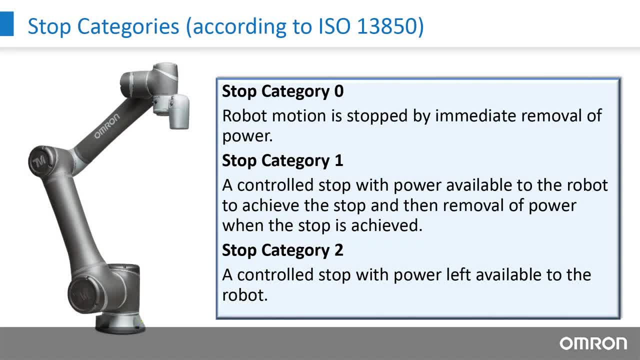 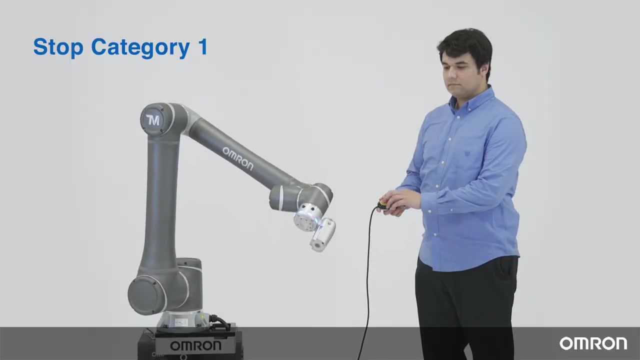 E-Stop is already in operation when the person comes in. In regards to the safety standard ISO 13850,, there are 3 stop categories With OMRON TM Robots. the emergency stop is Stop Category 1, where the robot's motion is stopped in a controlled manner with the power needed for that stop. 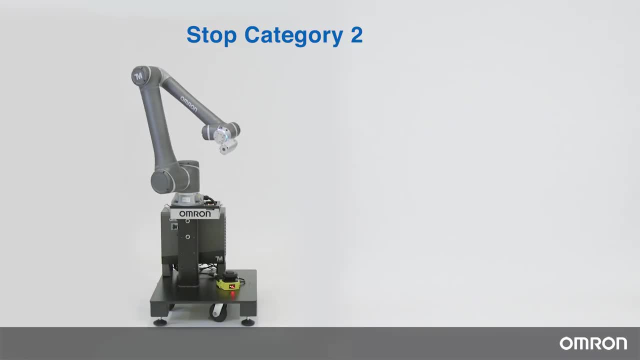 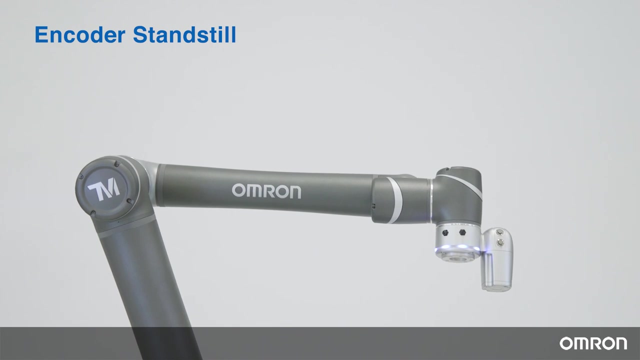 The power is cut when the stop is achieved. On the other hand, the protective stop is Stop Category 2, which is also a controlled stop, where the power is still available to the robot after the stop is achieved. There is also a safety function called Encoder Standstill. 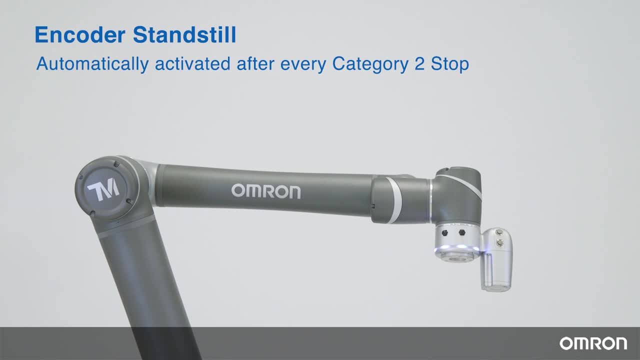 This safety function is automatically activated after every Category 2 stop. Encoders of each joint are monitored continuously to check if there is any unintended motion, until the robot is reset from the state of Category 2 stop. If there is any unintended motion, this safety function will trigger a Category 0 stop. 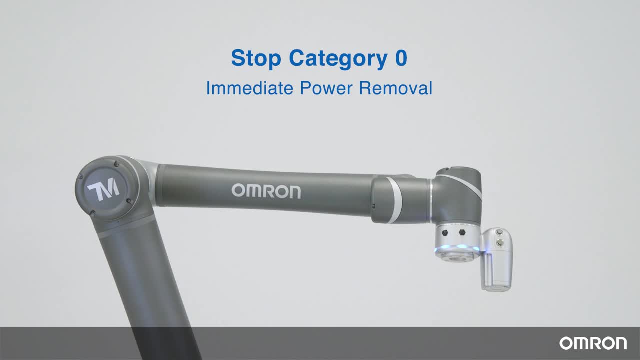 where the robot motion is stopped by an immediate power cut to the robot. When there is a discrepancy detected between two safety channels, the system will perform a Category 0 stop. also, This is the IO module in the control box of the OMRON TM robots. 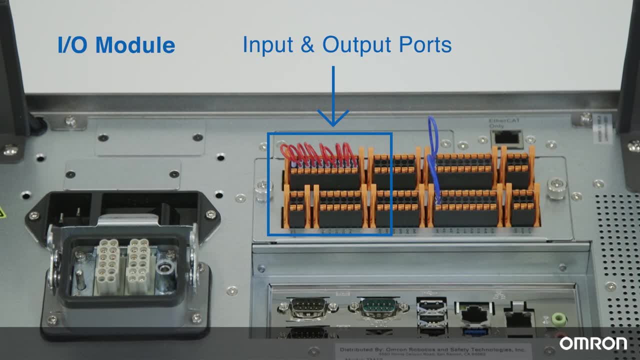 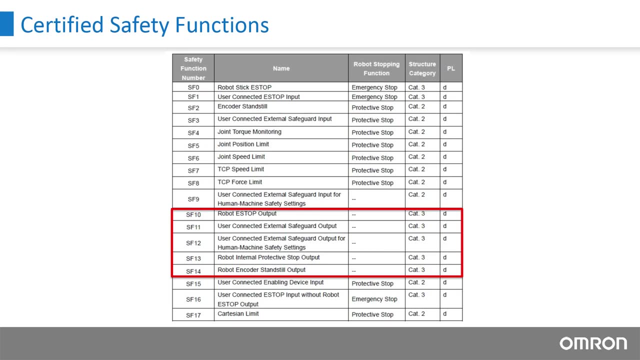 There are 10 safety input ports and 10 safety output ports. Safety Output Functions: Safety Functions 10 to 14 provide the safety output functions connecting to other devices for system integration. This means OMRON TM robots will constantly send out information about their status to other devices that need that information. 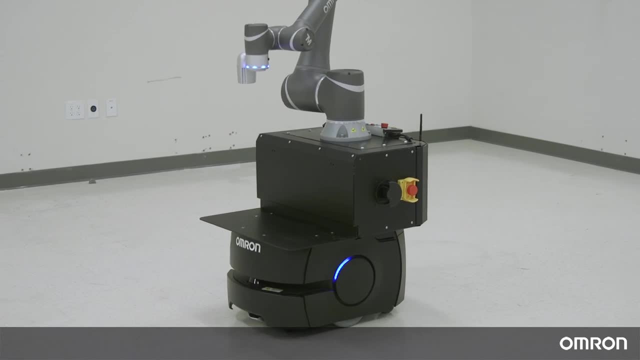 For example, many users are interested in mounting the OMRON TM robot onto a mobile robot so that it can autonomously move from one location to another. In this case, the mobile robot is connected to the OMRON TM robot. In this case, the mobile robot is connected to the OMRON TM robot. 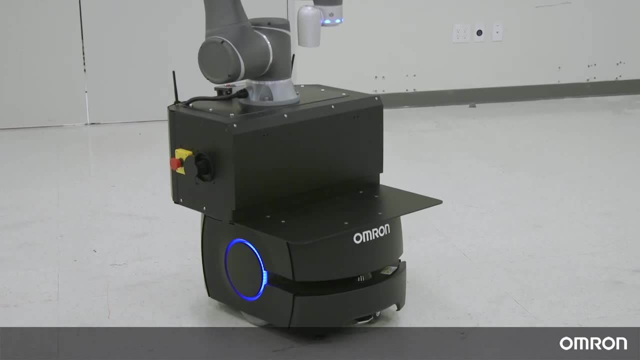 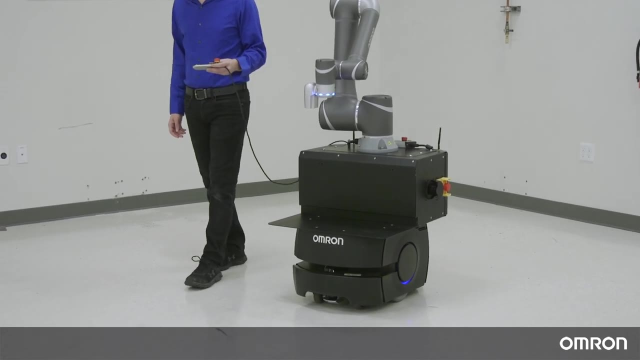 In this case, the mobile robot is connected to the OMRON TM robot. robot needs to know the status of the OMRON-TM robot to ensure the safe operation of the integrated equipment By connecting to the safety output if the OMRON-TM robot comes to an emergency.